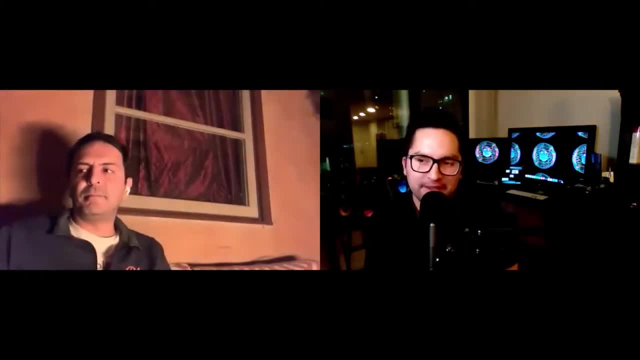 So I want to move a little bit into more interplanetary mission design, And one thing that I'm really curious about is the fact that when the mission designers go about designing, say, a mission to Jupiter or a mission to Neptune or Pluto, is that they do a bunch of flybys of the interplanets and other planets. 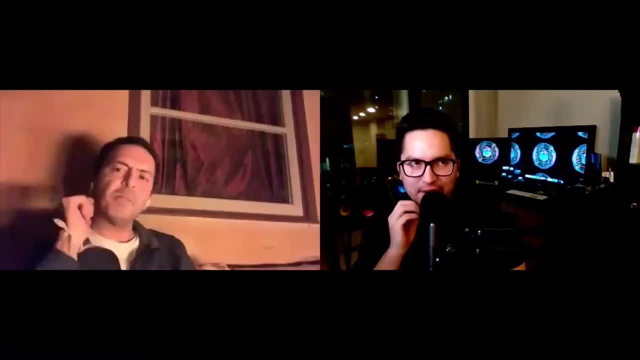 So I'm kind of wondering how that process goes of going through design, because I feel like there's so much freedom And the problem isn't very restricted, because I feel like you can do Earth, Moon, Venus, Mars flybys and you can just do a bunch of that. So I'm wondering, yeah, just how that process goes of actually picking these flybys. 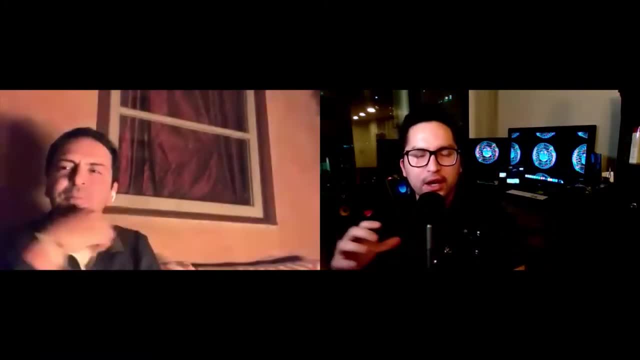 Sorry, could not hear the last part. You're wondering if you can pick what? Oh, just the process of how to pick these flybys, just because there's so much freedom to pick, just whatever you know. order of flybys like Earth Moon. 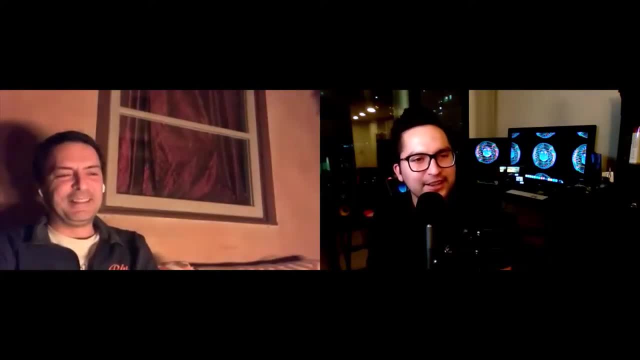 Earth, Earth, Venus, Mars, all that. Yeah, so there's two answers. The first answer is: there's no way to pick them, You just have to try them all, which is a bad answer. The good answer is that we have some idea. 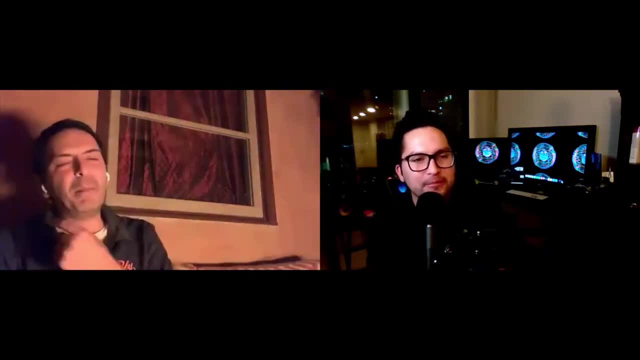 So the first one. you have probably heard that Tisserand, an old astronomer of the- Oh God, I forgot, I think it was the 17th century. Anyway, this person of last name, Tisserand, invented a criteria for when a comet flies by Jupiter. it sometimes explodes. 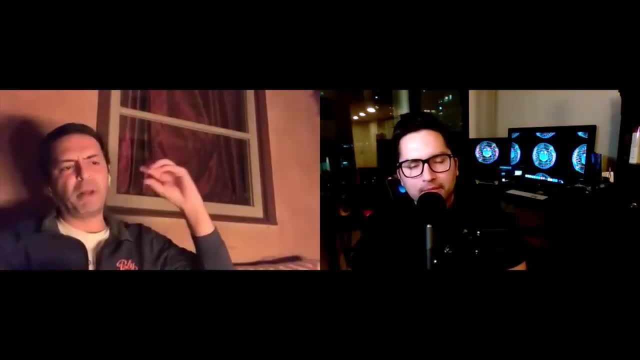 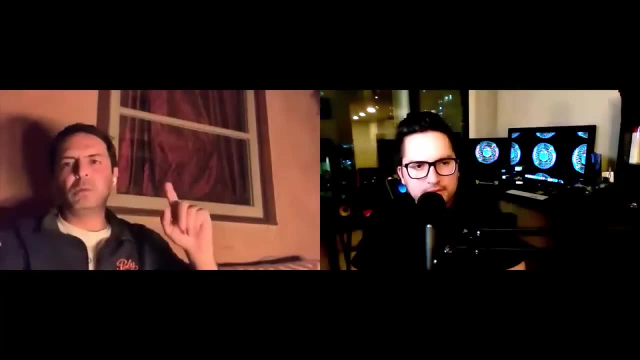 And then you had one comet, and then it passes by Jupiter, it explodes and there are several pieces of the comet. So at some point they didn't know which one which piece was from what comet. And this guy, Tisserand, developed a criteria. 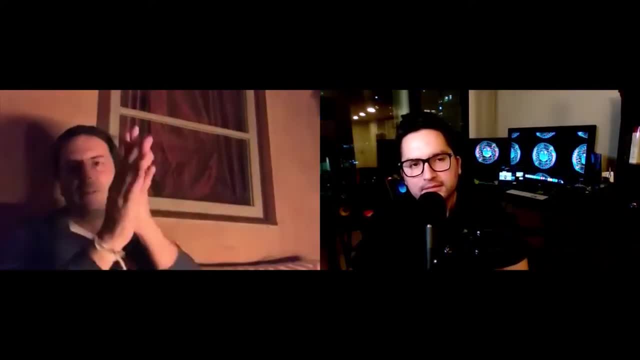 That said, okay, everything changes after the flyby and the subsequent explosion, But this one parameter doesn't, or doesn't approximately doesn't, And he invented this criterion that allows you to distinguish one thing before and after a flyby, So we use something similar. You can tell a priori what kind of change in your orbit you can expect from a flyby with each one of the planets or with any massive body. You know what is the mass of the body, depending on the incoming hyperbolic velocity that you have with respect to the body and the altitude that you fly by it. 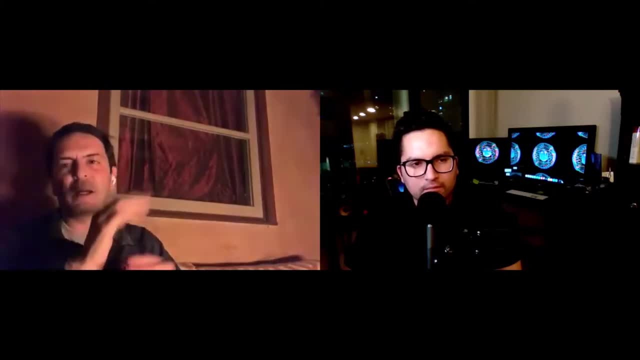 You know how much it would rotate your velocity vector relative to the sun or relative to the center of the trajectory that you're investigating, And you can bring these arguments into some sort of energy argument and finally develop something that is called the Tisserand parameter. 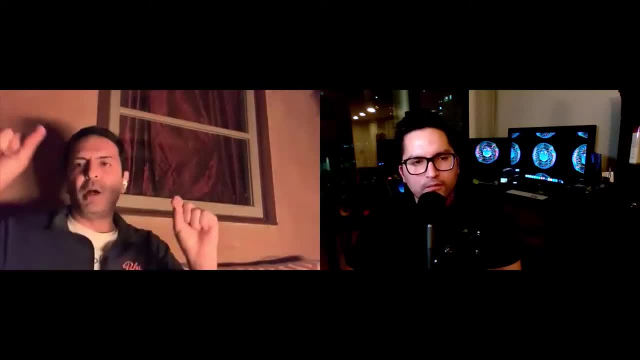 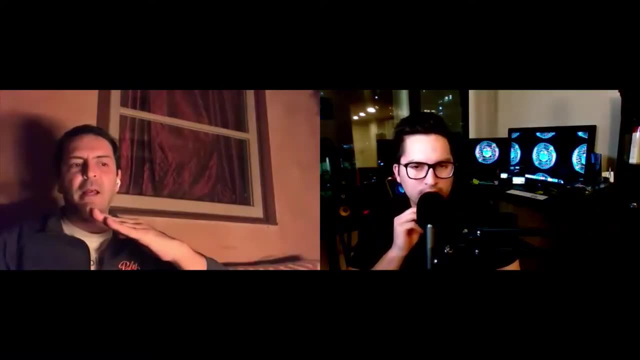 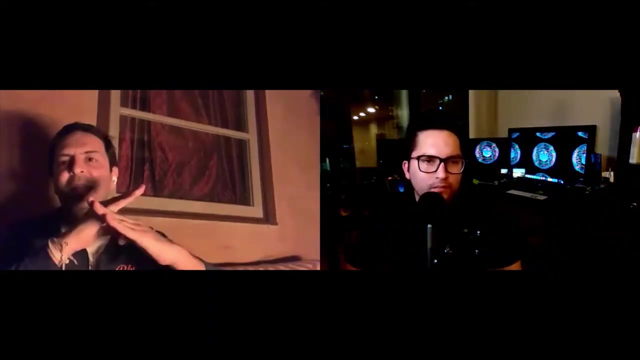 Which is inspired by this guy Tisserand. So you create these plots that tell you: okay, if I was at Earth with a V and V of so-and-so say, 9 kilometers per second, and I made a flyby, I could energetically reach, for example, Venus. 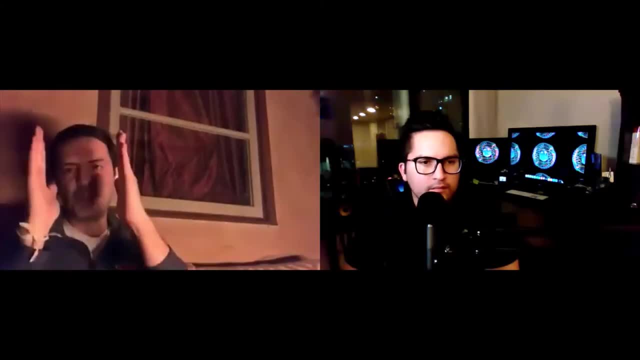 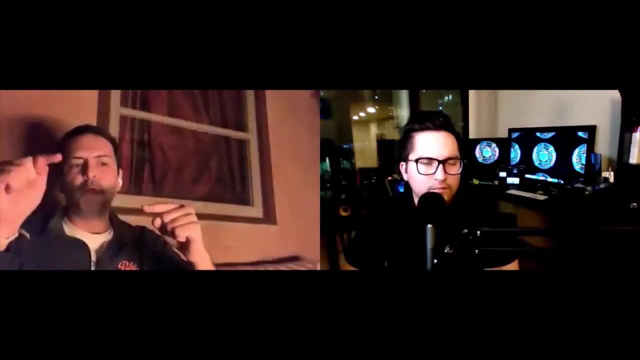 And if I did I could reach it approximately with this so-and-so hyperbolic velocity. And if I did, then I could reach Venus, And if I did, then I could reach, say, Jupiter, Or I could reach Earth back again. 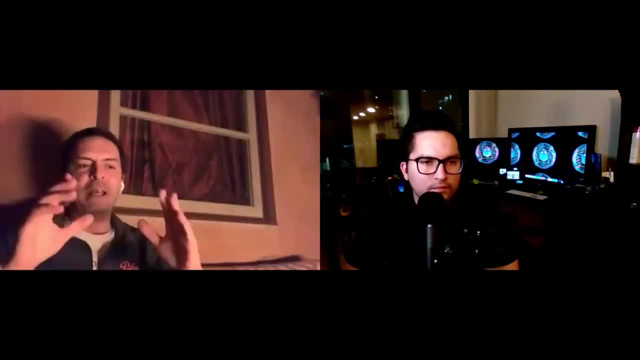 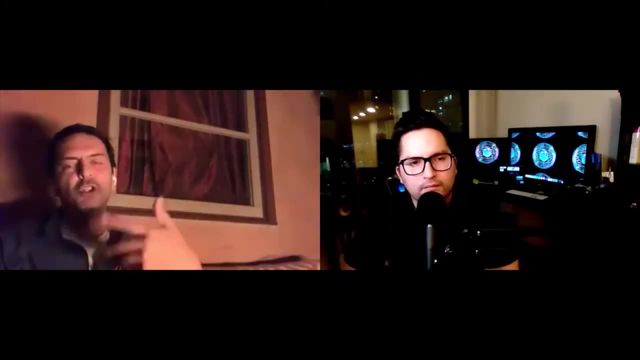 Or I could then orbit once and then reach Venus back again, And so we do have some guidelines on how to look. So you know that you are not in one flyby going to reach Uranus. You know that Because there's energetically not possible. Your time of flight is not sufficient, There's not enough energy in your orbit to have an apoaps that will intersect the orbit of the planet that you're trying to reach. So, when you have that Tisserand criterion, Your energy arguments, your charts that allow you to see flying by where, approximately? where could it take you? 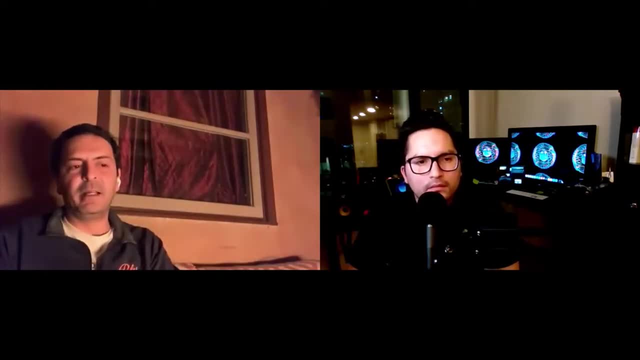 Then you have to deal with the second problem, which is the phasing. Namely, it is energetically possible to reach, say, Uranus with a flyby of Jupiter powered by Earth. It's energetically possible, We know that. 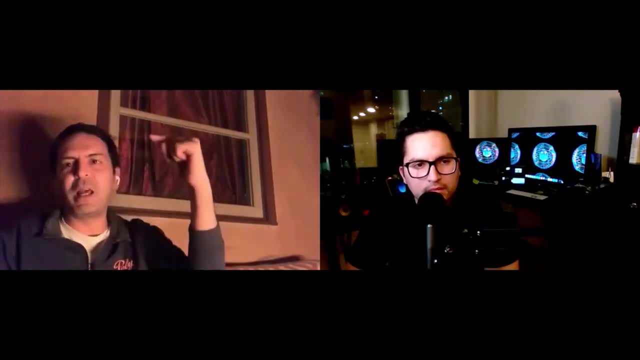 But that doesn't mean that Jupiter is going to be in the good location. So then you have to find it, And unfortunately, I mean there are some approximations. You can assume that all the planets move in a circular orbit, which is not too bad of an approximation. 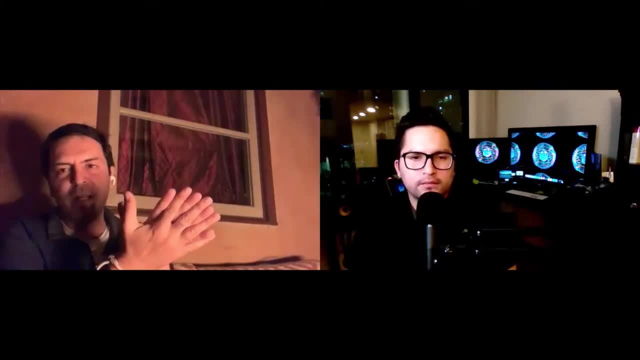 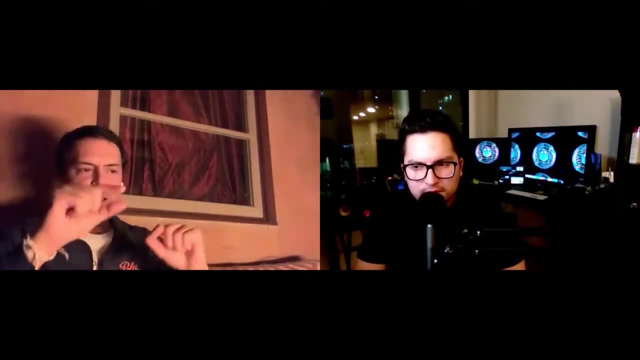 That they are coplanar to the ecliptic- which they are not- And say, OK, I'm going to start with circles, I'm going to get some sort of timing, Then I'm going to from the circle solution that is coplanar, I'm going to add some. 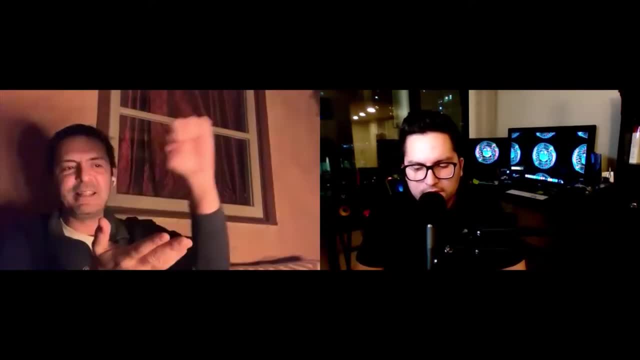 I'm going to add some out-of-plane full ephemeris to what we have done at NABLA Zero Labs to search it in full ephemeris. So it's not high fidelity but it's full ephemeris very fast. 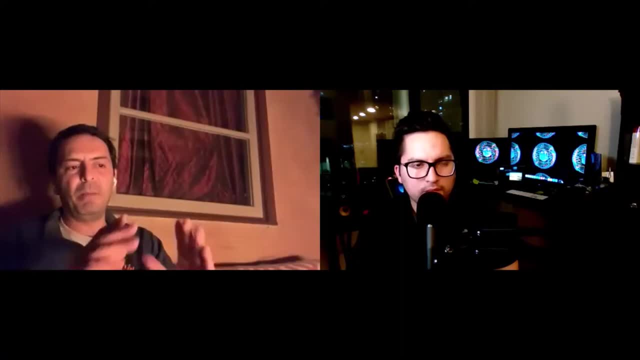 And honestly, in my experience, I very quickly use a discernment-like criterion to discard what I cannot search. I say, OK, I'm not going to consider, for example, Mars, I'm not, I'm going to consider more than two Venus flybys. 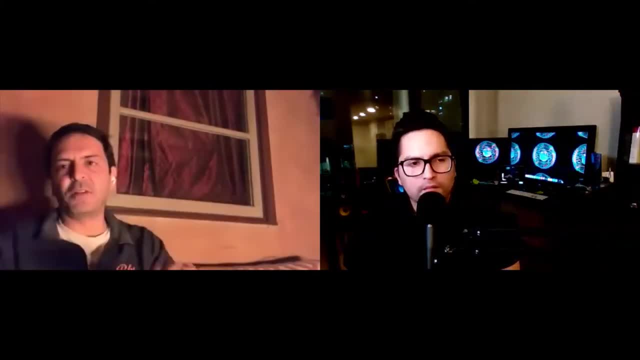 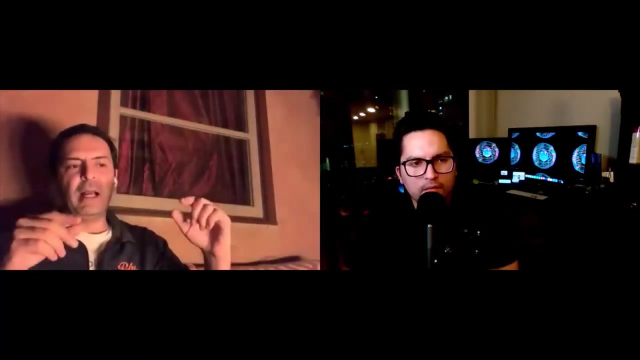 And I'm not going to consider Saturn. Everything else is on the table. And then I just set up my time of flight bounds, I say I want to depart from Earth with the launch vehicle I know- Neptune within 20 years, And then I just filter what I'm not going to do. 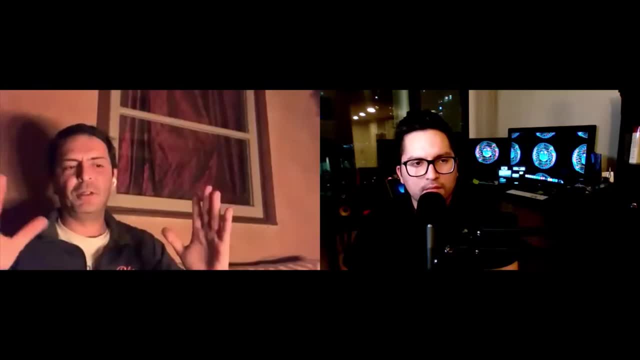 And just start a very coarse search throughout the rest of the domain. I leave it running for three days with several computers and just to get an initial peek at what's out there, And then, once you have this very broad search after some high-performance computing, 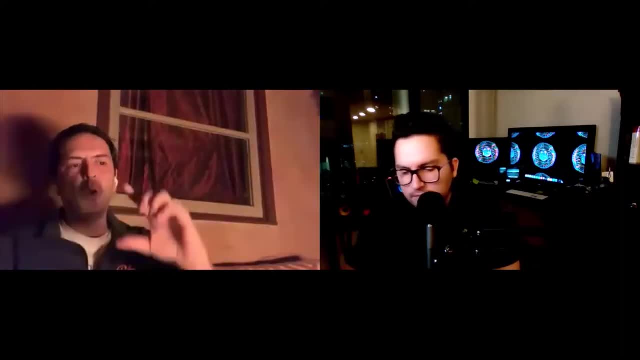 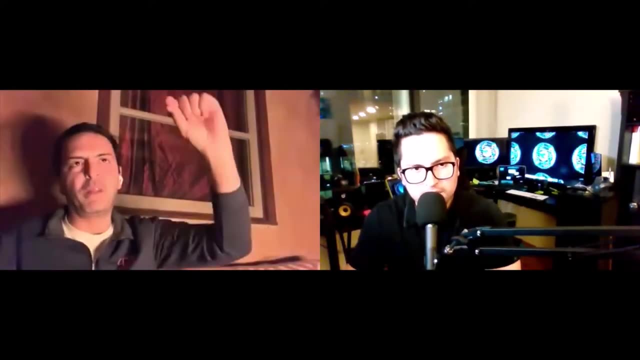 then you start zooming in some regions and say, oh, look, my Earth, Venus, Earth, Jupiter, Neptune are looking good for the 2040 decade. And then you start fine-tuning it. You say OK, oh, you see the flyby. 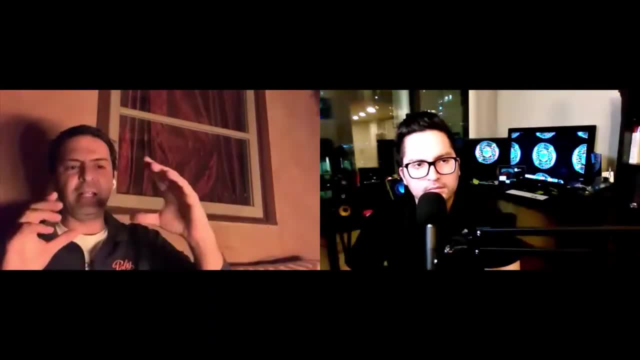 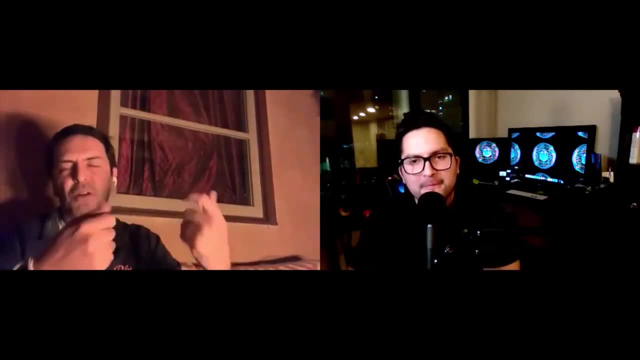 It starts getting out of focus. It's face here, It starts getting in face here And then you start pinning it down. But at the end of the day you just have to run a bunch of studies Again. you can study some energy arguments to know what not to do. 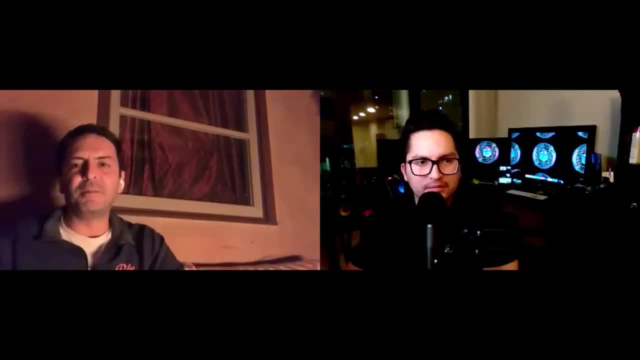 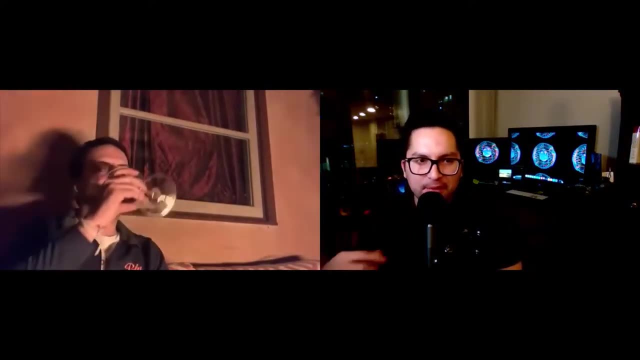 But it's artisanal and computationally a very expensive process. OK, so once you have kind of some candidates, say you're doing a mission to Neptune, and you have some candidates of trajectories that do a certain amount of flybys, So 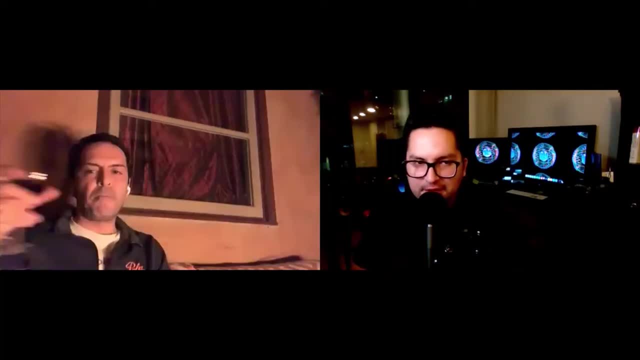 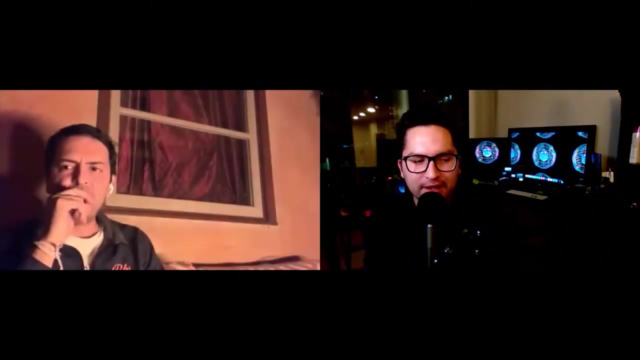 How do you go about then refining these trajectories to make them higher fidelity? So, as far as you know what maneuvers you're going to do, as far as propagation, do you use a patch conics way of propagating methods? Yeah, How do you start refining these trajectories once you found that these are feasible? 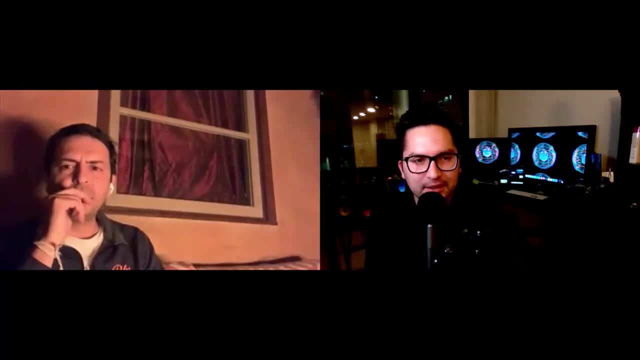 And I want to look more into these. Definitely, You always start with the best friend Of the mission center, which is a Lambert solver. The orbital boundary value problem is the name of the problem that connects two points in a space with a single point mass. 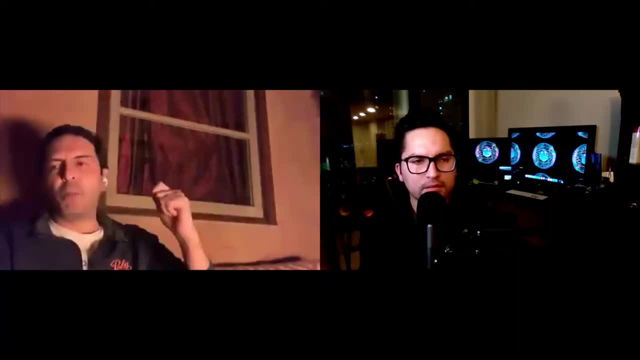 So it's a two body problem solver. It connects two points in a space in a pre-specified time of flight. Given the two position, it gives you the two velocities that will make that conic. expand the two positions in a prescribed amount of time. So you get that solution. If you have to make a flyby, then what you need to do is: okay, I go from, say, Earth to Jupiter, I solve a Lambert arc, I get the velocity of Jupiter when I came into Jupiter and then say: you want to go Jupiter, Neptune. So then you solve a Lambert from Jupiter to Neptune, and that will have. so you have now an incoming V infinity at Jupiter and then outgoing V infinity from Jupiter. And you have to, Because energy is conserved during a flyby relative, flyby body. 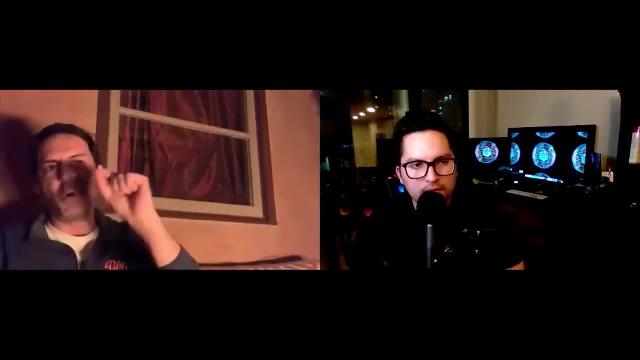 So you know that the energy of an orbit, so energy- is the square of the velocity divided by two, minus gravitational parameter divided by the distance. And because the velocity is conserved there, the only thing that can happen with a V infinity vector is that it can rotate. 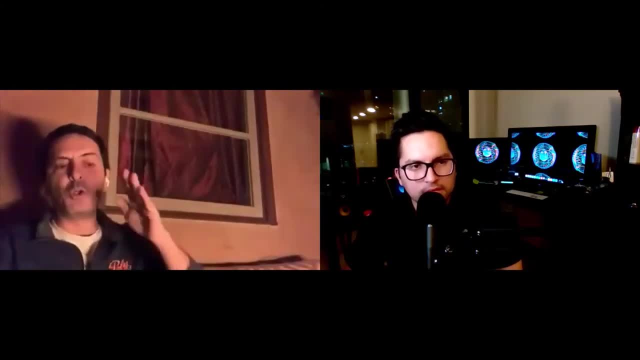 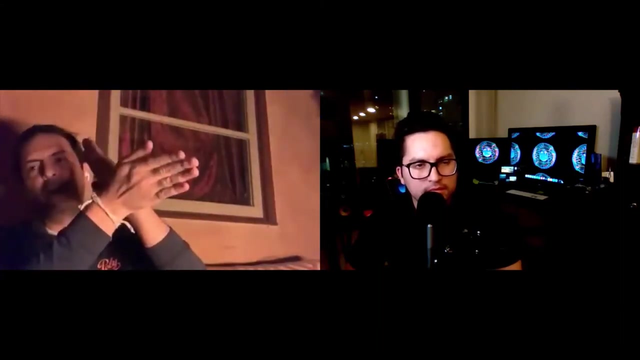 But it cannot change it. It's magnitude. So you need to have the magnitude of the incoming V infinity be the same as the magnitude of the outgoing V infinity, And then you have to evaluate the angle by which the other, by which you have to rotate the first one to get the second one. 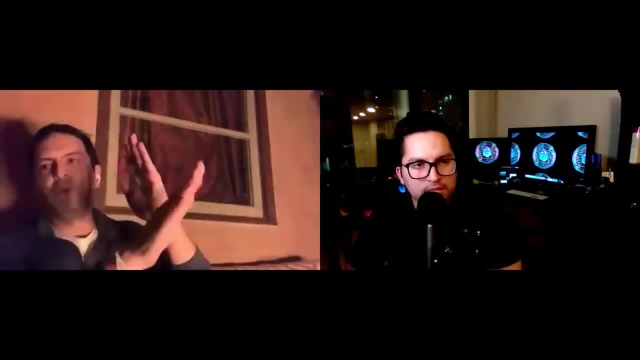 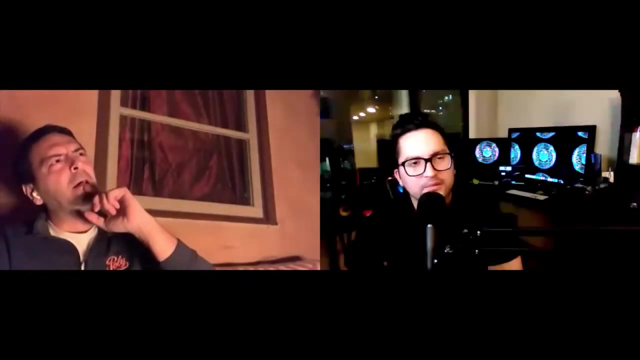 And that angle has to be compatible with the flyby altitude. There's another formula that allows you to compute the flyby altitude, given an inbound and outbound V infinity vector. I forget it, But It's again like: how about V infinity minus inbound V infinity? the magnitude of that equals twice V infinity divided by one, plus twice V infinity divided by mu. I think something like that. 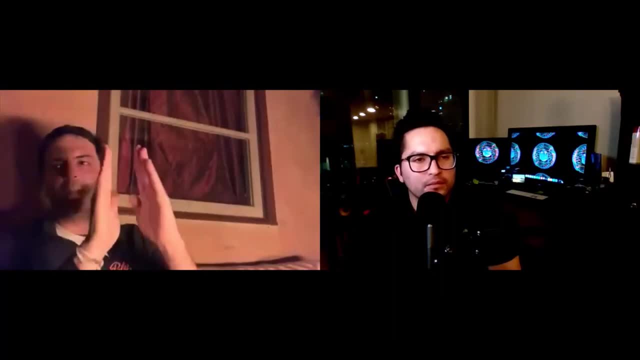 So with that, you, you get the minimum flyby. And then you are like: okay, I got my earth to Jupiter. It has a given V infinity vector. I got a Jupiter to Neptune: It has another V infinity vector- The magnitude of this one. 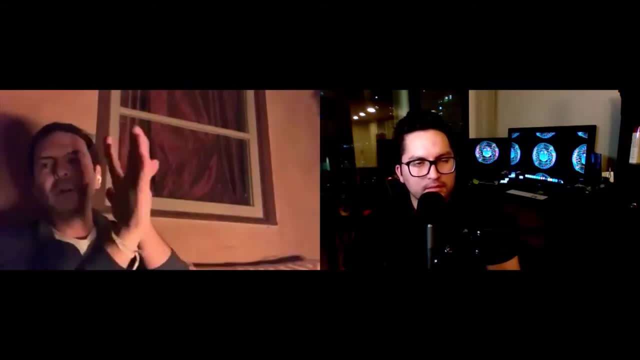 Is the same as the magnitude of that one, And the angle between them is Within the altitude that I'm willing to go say is greater than 200 kilometer altitude. So then you, you get this parameter. So that is called the patch conic approximation. 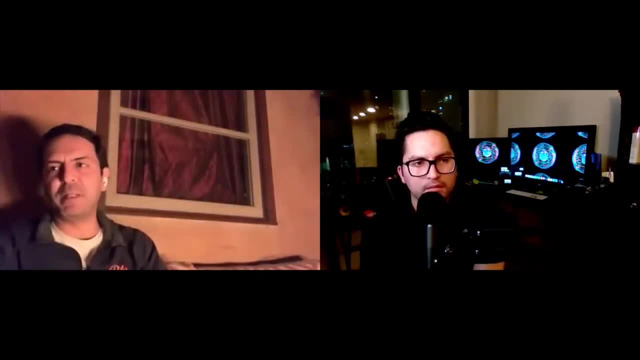 And now, when you have those two, you can say, okay, now I want to solve it in full fidelity. So for the flyby, given the inbound and outbound V infinity, You can calculate an approximate, What we call a full fidelity state relative to the flyby body. 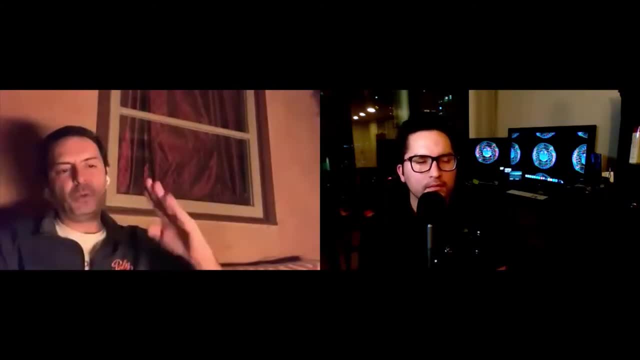 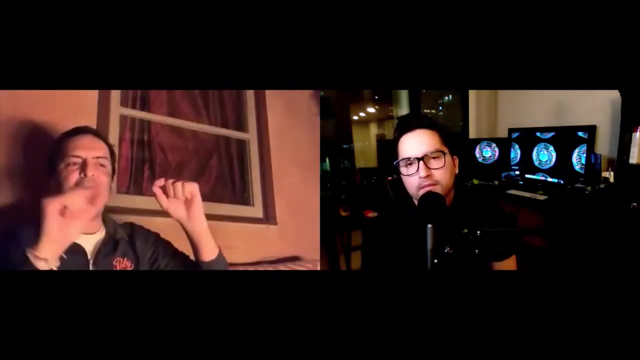 You normally calculate the B plane parameters, But you you can calculate the position and the velocity of the spacecraft relative to the flyby body And you convert that state onto the B plane target And then you now have an initial condition, a B plane target and the final condition. 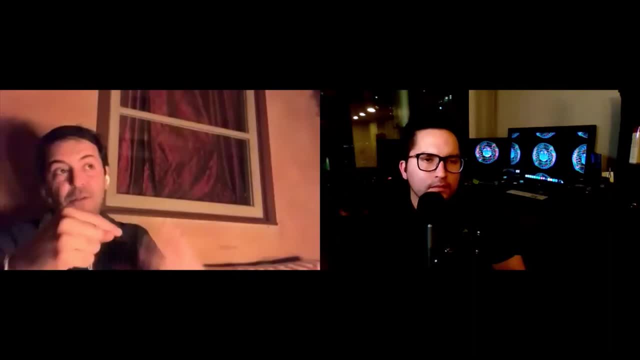 And you use that as the initial guess, As the initial guess, As the initial guess, As the initial iterate For a full fidelity. Multiple shooting, collocation, What have you? But that is normally the process: Lambert C3 matching or V infinity matching. 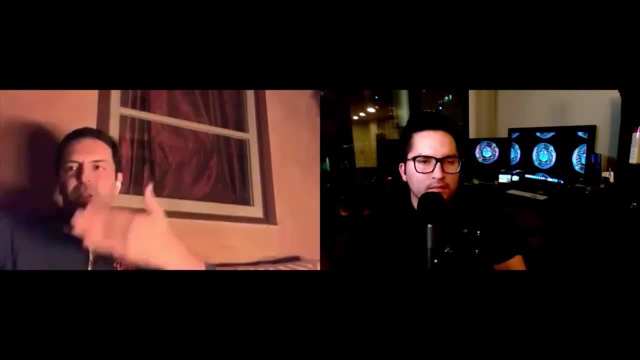 Approximating the states, Getting the B plane targets And passing those on to the full fidelity solver that uses full ephemeris. Calculating the launch window is a little bit different Because you only have an outbound V infinity vector And that one you just have to. 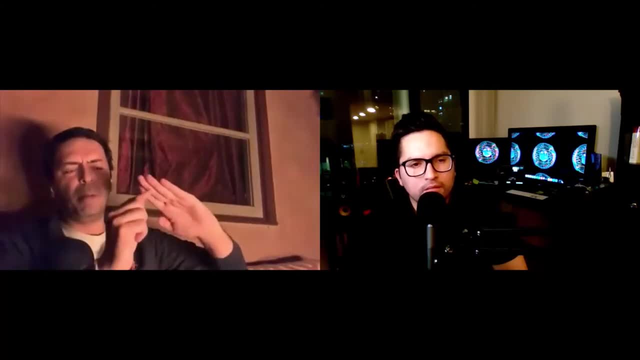 Start in a circular orbit around Earth And pick a point in that orbit that will result in the same outbound V infinity vector. So you get the right ascension, declination and magnitude of the outbound asymptote And you just find the circle at which you are applying a delta V. 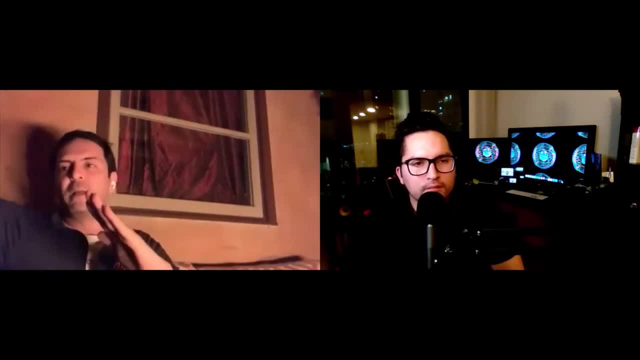 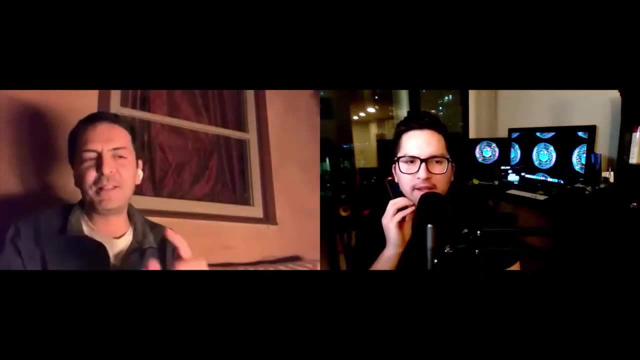 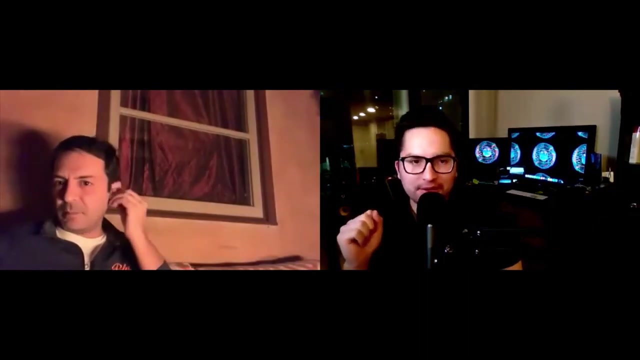 You will get that outgoing hyperbola, And then you that's how you go, And then you just target coming into the next one with another B plane, And off you go. It's easier said than done, though, Yeah, So can you talk a little bit about as far as the patch conic sense? 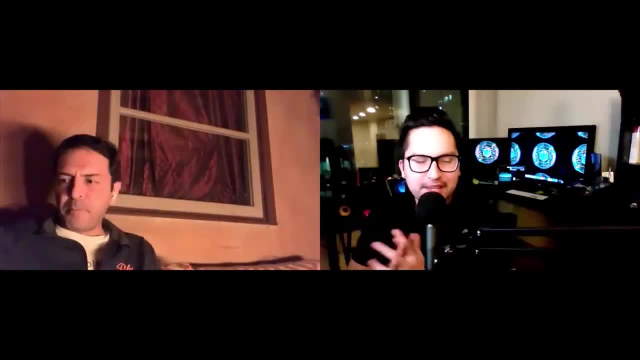 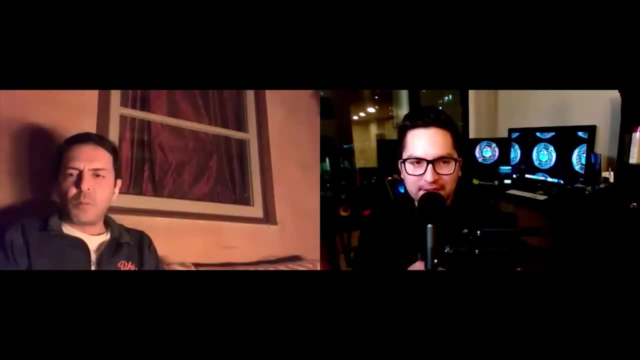 So doing center switching and sphere of influence. So say, as you're coming into Jupiter, At what point do you want to say that I'm no longer in an elliptical heliocentric orbit? I am now in a hyperbolic Jupiter orbit? 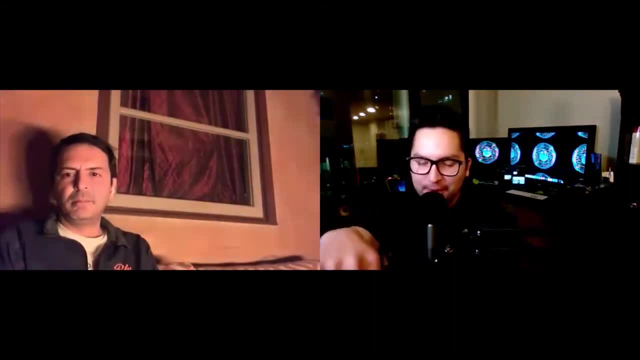 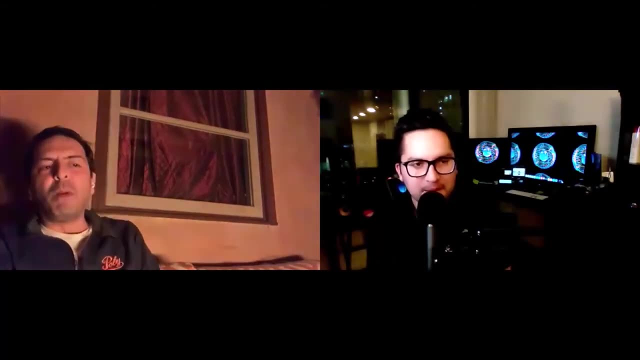 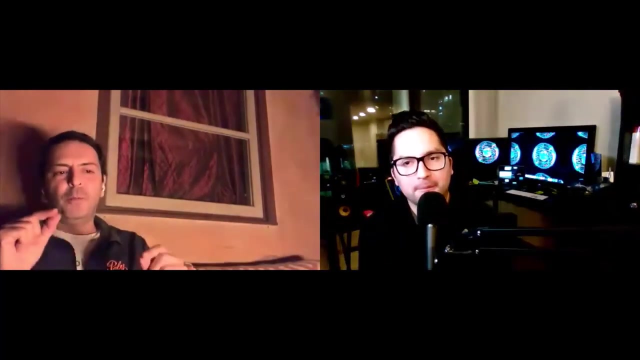 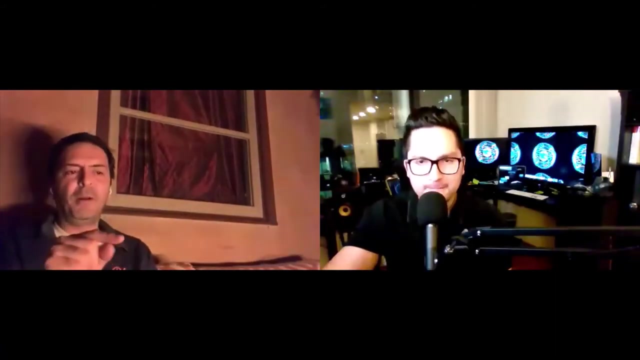 And then, once you come out, I'm no longer in this hyperbolic Jupiter orbit. I'm now back again To a heliocentric elliptical orbit. Yeah, normally when you, the answer is both simple as complex. When you want to consider Jupiter as a flyby, in the case of Jupiter in particular, 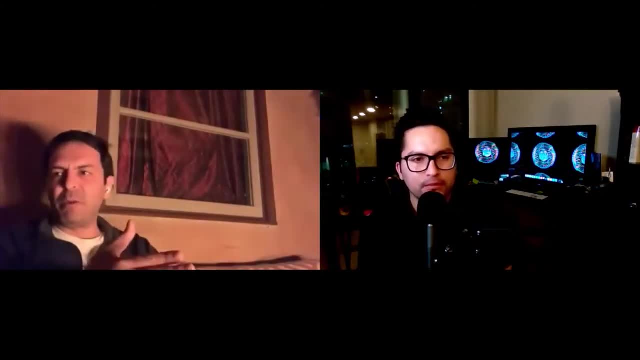 You would always do it when you are within its actual sphere of influence. When you- which you can calculate in my case, to me Jupiter is a two million kilometer kind of deal. If you are three million kilometers from Jupiter, I normally do not enter the sphere of influence. 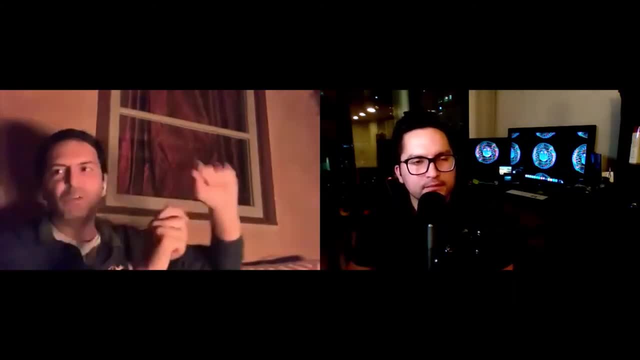 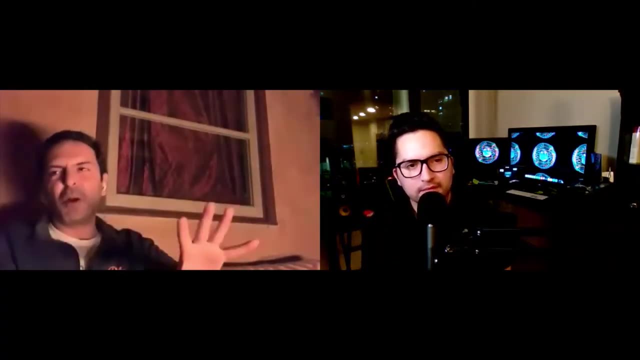 I normally don't consider it as an individual point, mass subject to the little moons orbiting. I just consider it a like a barry center with all the matter. we are in center at three million kilometers, just as a rule of thumb. But if I'm considering as a flyby is normally because I'm closer to it, like, say, two million kilometers and closer. 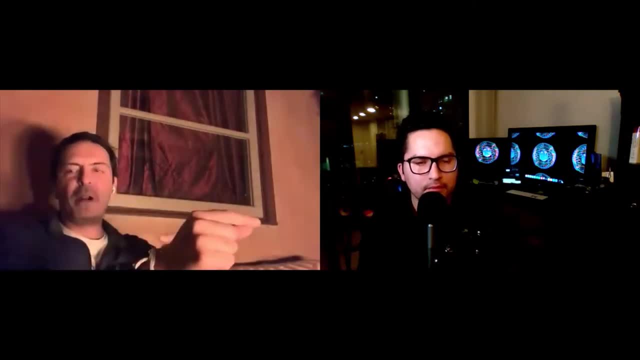 Then it is just, I put the The pointer, and when I get to that three, two and a half million kilometers distance, Then I trigger the center switching and precisely what you said happens. You are a heliocentric, elliptical, not necessarily elliptical. 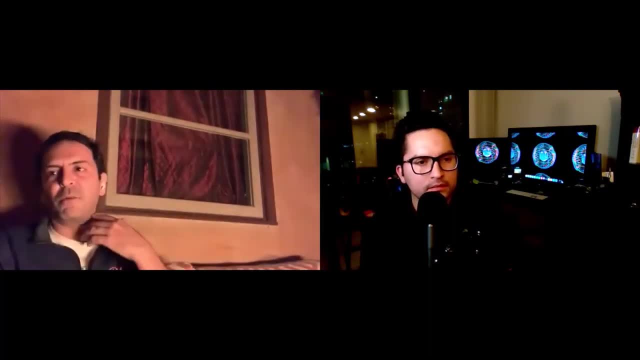 You can have a non elliptical, like New Horizons, For example. it had a non elliptical orbit relative to the Sun. It was like a screeching when the spacecraft took off. Heliocentric, The big plane, Which are approximately linear relative to the velocity at the beginning. 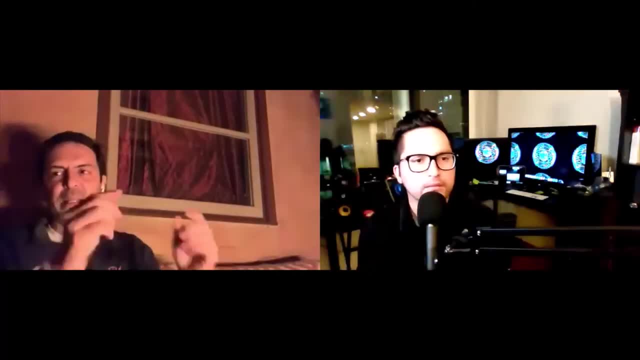 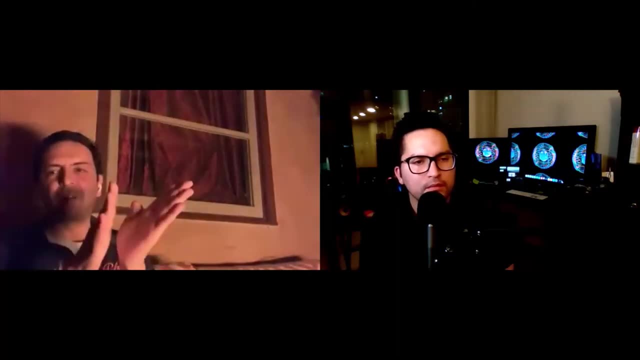 That's why we use them, because they are not as wildly varying as the norm. If you just compute the distance to Jupiter, that's obviously a quadratic. because you have a vector, another vector, You subtract them and you take the norm, which is a square root.